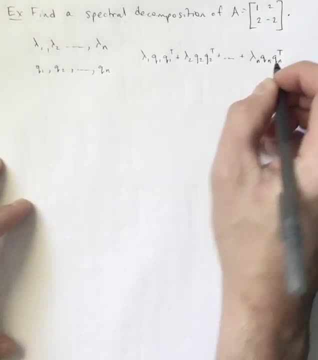 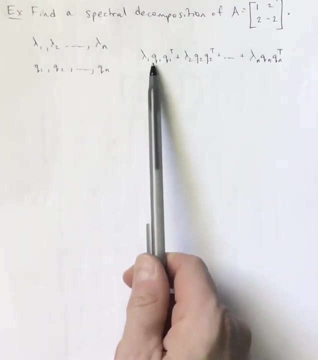 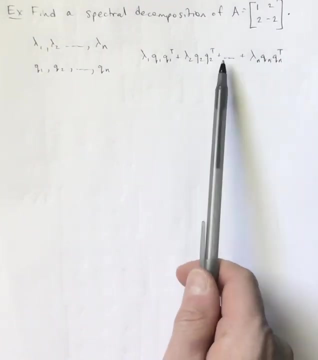 linear combination as shown. So remember that q1 through qn are going to be n by 1 vectors. So q1 times q1 transpose will actually give me an n by n vector. So each one of these are n by n vectors. 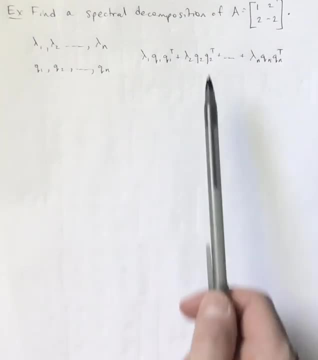 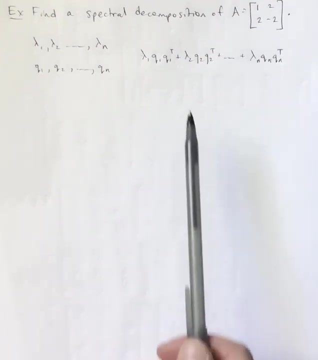 The lambdas, of course, are the scalars, which are real numbers. So we will get a linear combination where the coefficients are the eigenvalues and then these matrices that we get serve the role that I mentioned at the top of this video. So let's see how to do that for this. 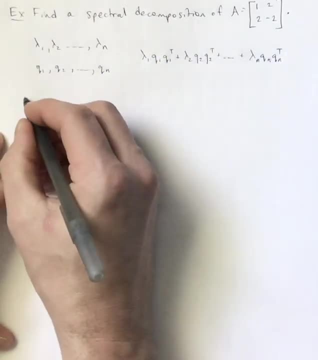 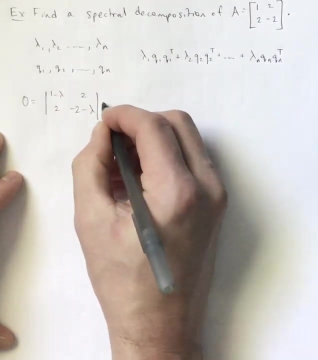 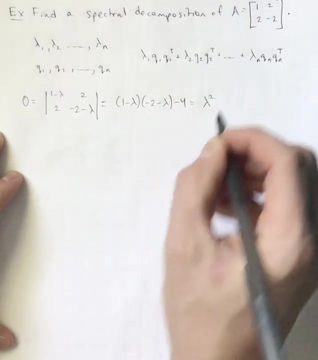 We do need to find, obviously, the eigenvalues for this first. So let's start by setting that up in the way that we do that. So there's two eigenvalues. So what I end up getting when I multiply all this out, the characteristic polynomial is lambda squared. 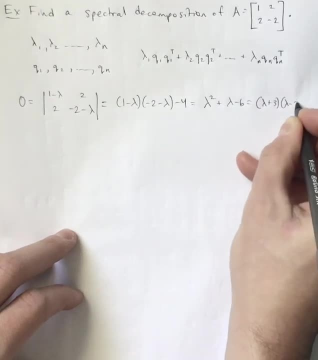 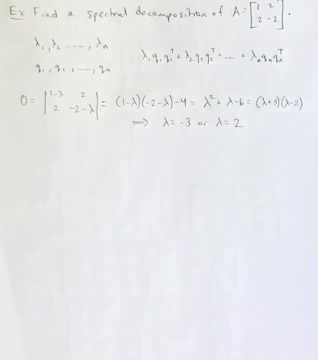 plus lambda minus 6. And that is lambda plus 3 times lambda minus 2. So I get lambda equals negative than 3 or lambda equals 2.. Those are my two eigenvalues. It doesn't really matter which order I do these in. 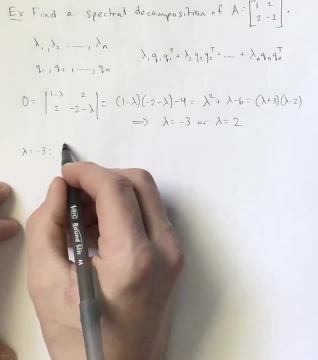 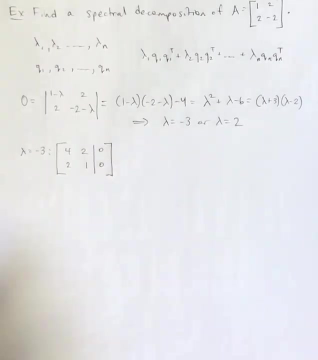 start with. lambda equals negative 3.. If I put that in right here, I'm going to get 4, 2,, 2, 1, and then, of course, put the zeros on. since I'm solving that homogeneous system, Notice that the top row is twice the bottom row, so using row operations. 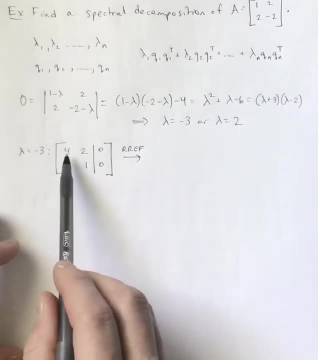 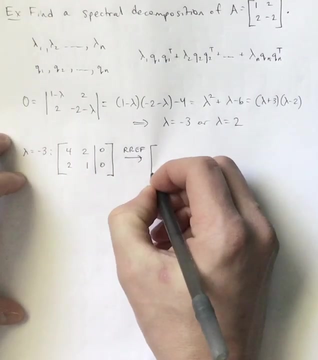 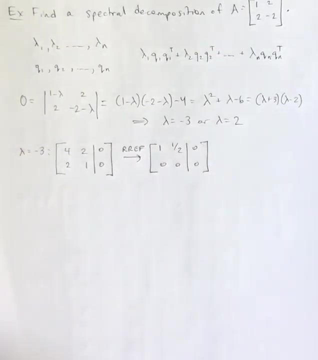 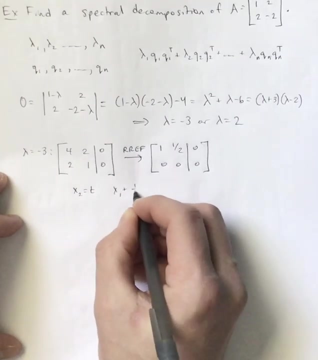 one of those rows will zero out, and in fact we could just make this one zero out and we could multiply the top row by one-fourth. That way we'll get a leading one right there. So this is going to be the RREF for this matrix. Now, x2 is our free variable, and x1 plus half of x2 is zero. That's. 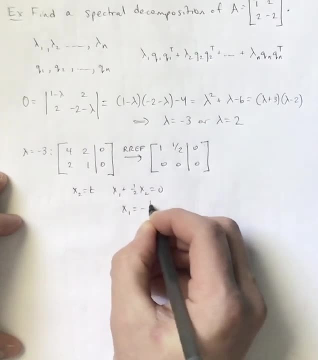 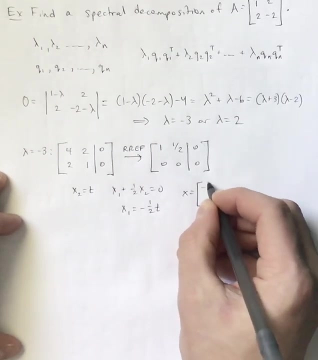 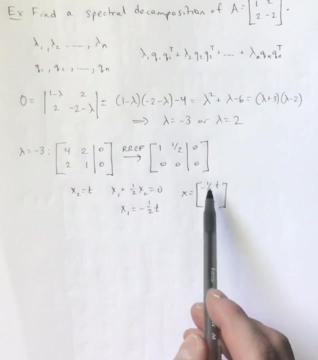 that top row, and of course that means x1, would be negative one-half t. So my matrix, or my vector rather, is going to be minus one-half t t. Now, if I took the t's out, that would be fine, I would have. 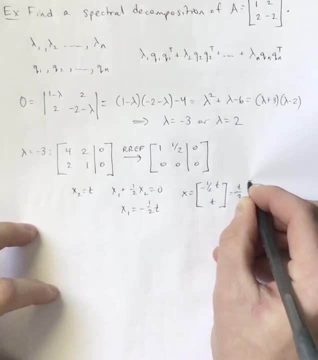 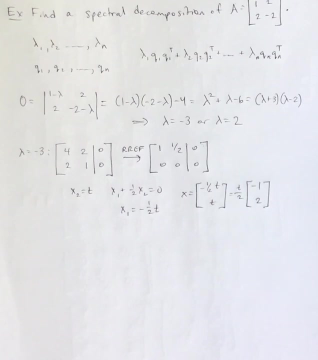 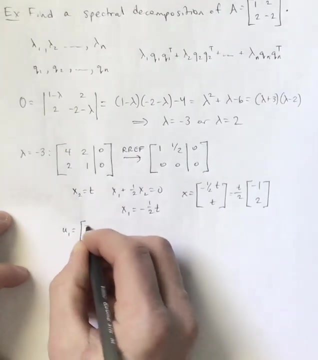 negative one-half 1, but I'll go ahead and pull out t over 2, and that way what I end up getting is a vector with integer coefficients which is much easier to work with. So that is going to be my u1, but, as we saw in the last video, if the eigenspace has, 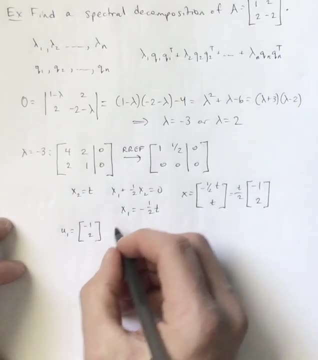 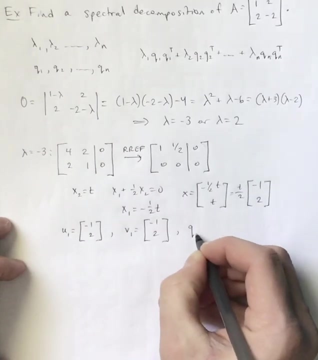 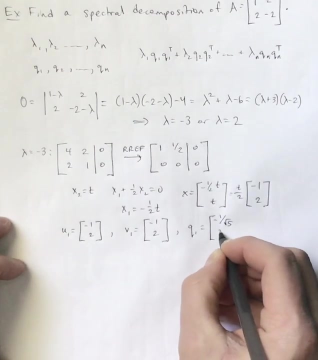 a single vector as its basis, then not only is u1 that, but v1 is that as well. And then to get q1, we will just normalize v1.. So the magnitude of v1 is root 5, so I'll get negative 1 over root 5,. 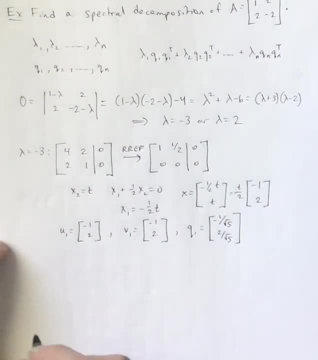 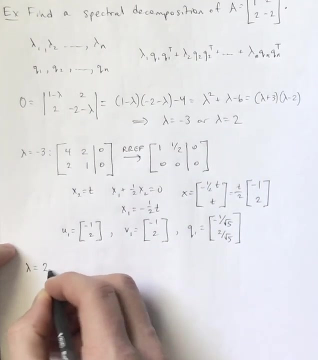 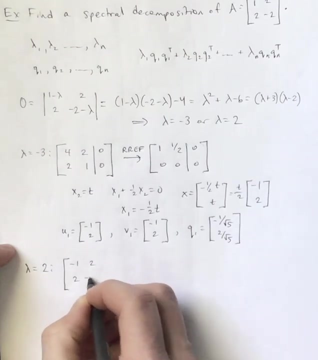 2 over root 5.. All right, so that's one of the q's in the spectral decomposition. Let's find the other one. And so for lambda equals 2, if I plug that in here, I'm going to get negative 1, 2, 2, negative 4.. 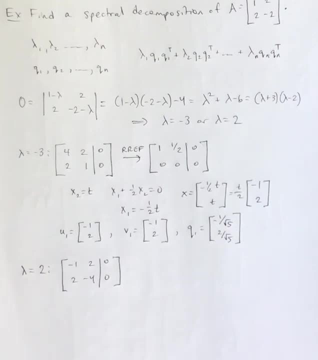 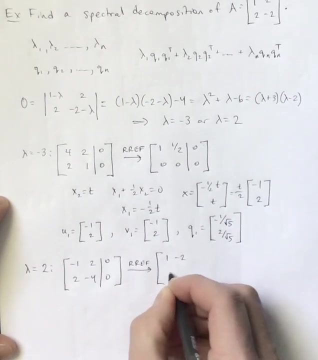 And you'll notice that the bottom row is twice actually negative, 2 times the top row. So this one will zero out and then if I just change the sign on the top row to get a leading 1,, this is the RREF for v1.. 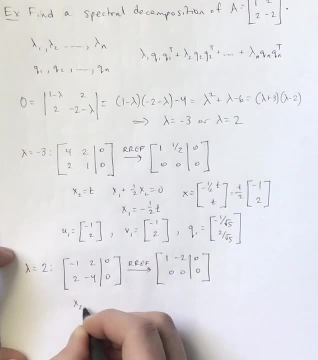 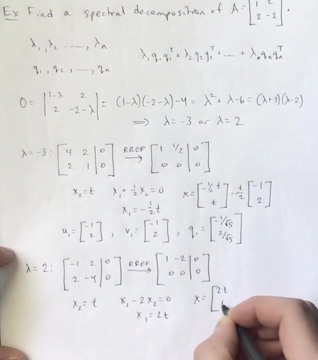 That matrix And so if I again have x2 be equal to t, then that equation is: x1 minus 2x2 is 0, which makes x1 2t. So in this case x is of the form 2t comma t If we factor the t out. 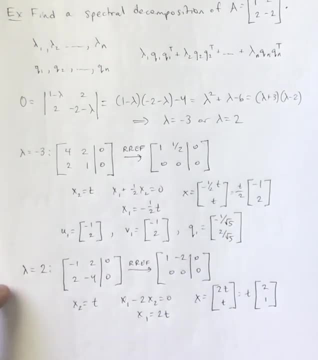 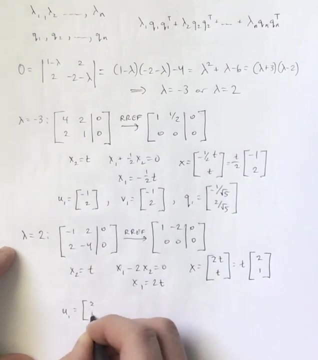 we have 2, 1.. So again, there's just a single vector in that basis, And so therefore, v1 is that vector, v1 is that vector, And then q- actually I guess I should say 2.. 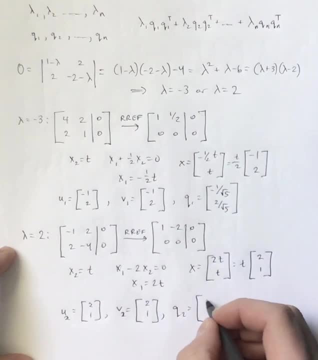 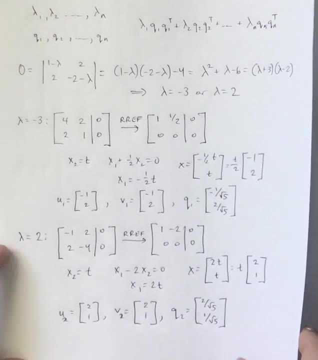 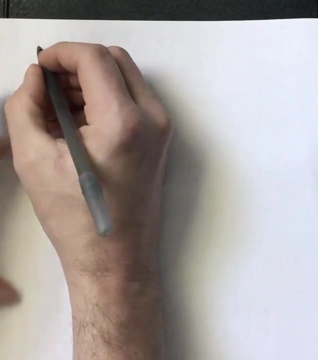 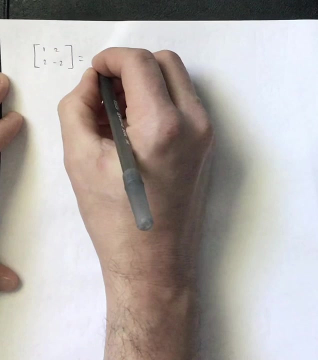 q2, this again has a magnitude of root 5.. So we'll say 2 over root 5, 1 over root 5.. So now that we have the q's, let's go ahead and find that decomposition, The decomposition for this matrix. Remember it should have negative 3 as one of the coefficients. 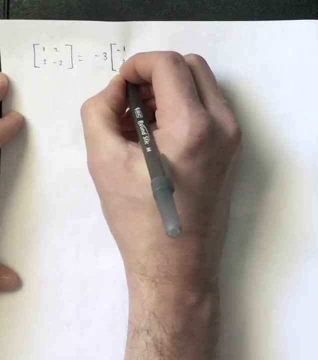 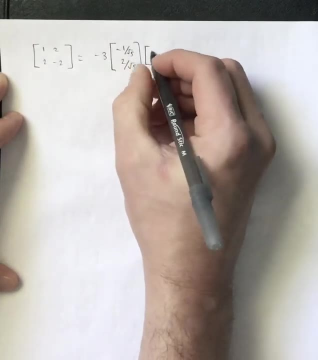 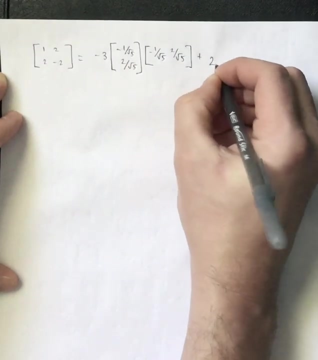 And in fact, negative 1, 2 was the- or sorry, negative 1 over root 5, 2 over root 5 was the vector. So then we're going to multiply by its transpose And we're going to do a similar thing. 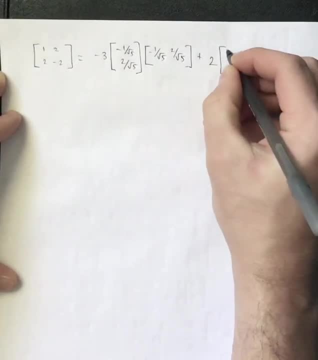 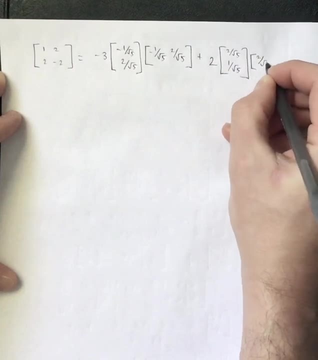 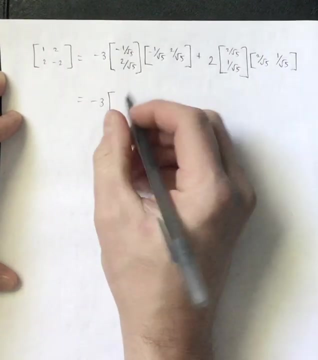 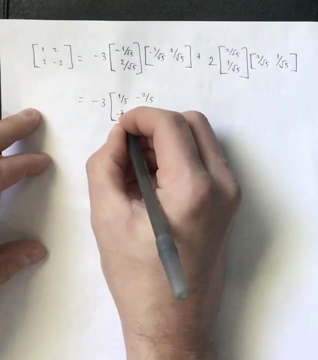 for lambda equals 2.. We're going to multiply that by 2 over root 5,, 1 over root 5.. And then that by its transpose. So this matrix is going to be: 1, 5th, negative, 2, 5ths, negative, 2, 5ths, 4, 5ths. 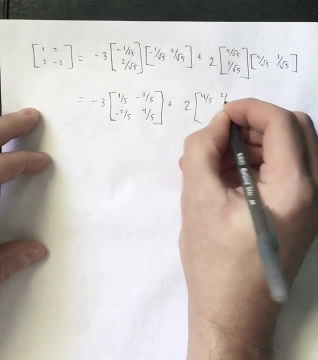 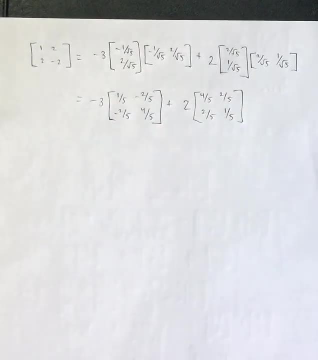 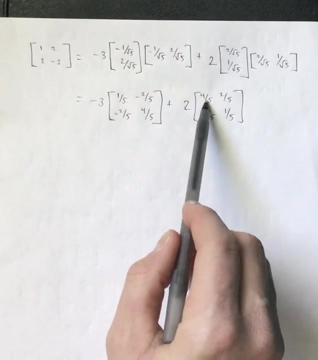 And this matrix is going to be 4- 5ths, 2, 5ths, 2 5ths, 1, 5th. And we can do a quick check just to verify that this decomposition is in fact a decomposition Negative: 3, 5ths plus 8, 5ths is 5- 5ths, which is 1.. 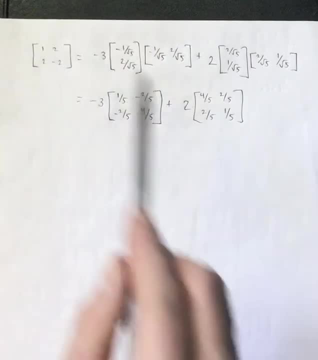 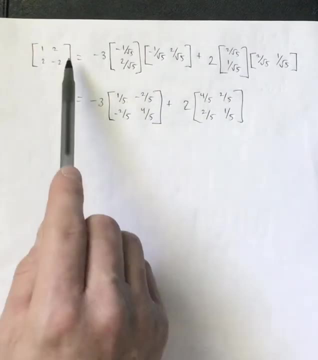 6 5ths plus 4 5ths is 10: 5ths, which is 2.. 6 5ths plus 4 5ths again is 2.. And negative 12 5ths Plus 2: 5ths is negative 10 5ths, which is negative 2.. 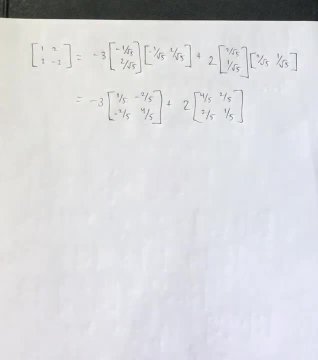 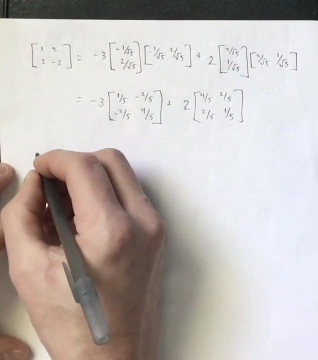 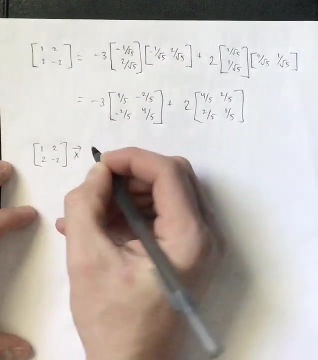 So this is in fact a decomposition. And now what we want to do is we want to see what the significance of this is, Because this is our answer. But what does a spectral decomposition tell you? Well, if we were to apply this matrix A by any 2, by 1 vector, let's just say x. 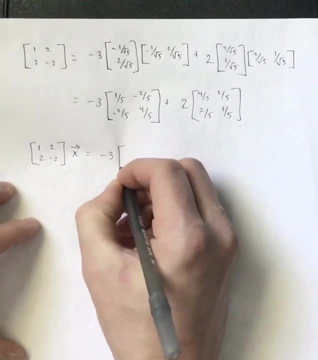 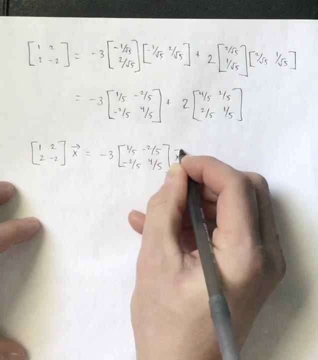 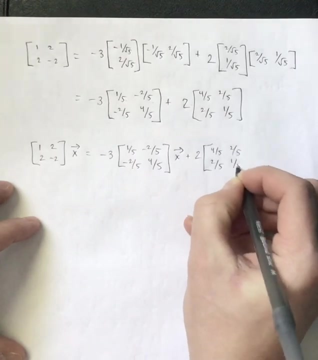 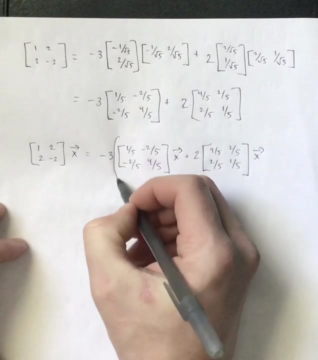 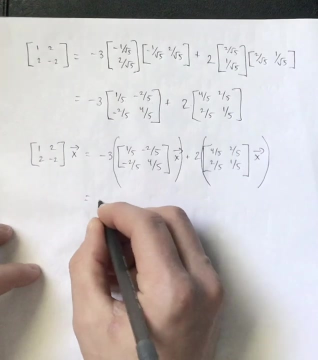 Then we know that that will be the same thing as negative: 3 times this matrix times x, Plus 2 times this other matrix times x. Now, if I look just at this part and the same part on the second one, What that's going to end up being is: this is the projection. 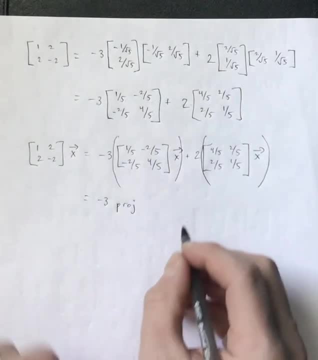 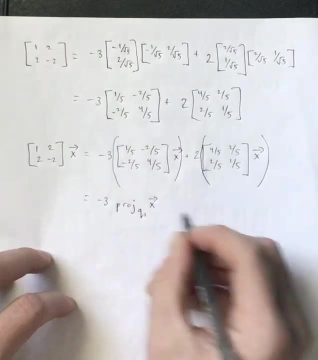 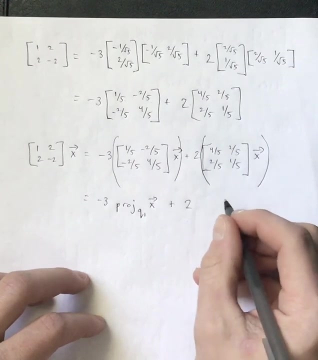 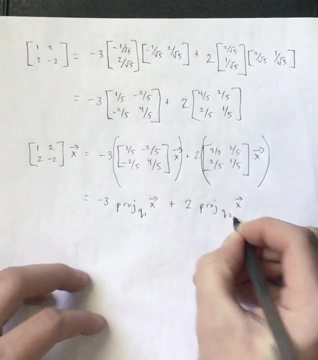 Or this will be the same thing as the projection of x onto q1.. I'll compute this in just a second to show you. And then this will be 2 times the projection of x onto q1.. And then this will be 2 times the projection of x onto q2.. 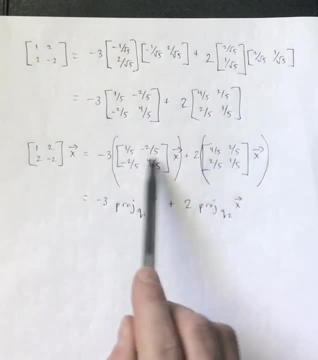 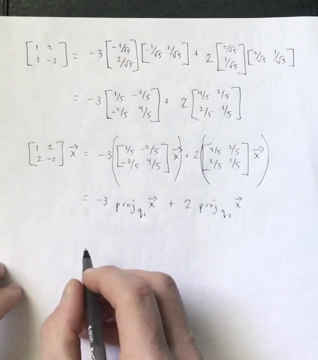 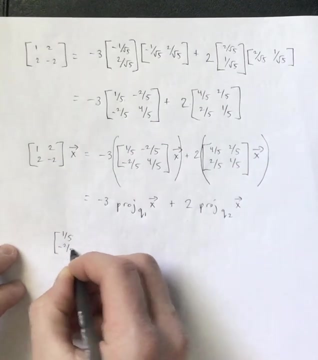 Alright. so it essentially gives you. multiplying this matrix by x gives you a vector in the direction of the two basis normalized basis vectors. Just to convince you of that. So let's say that I did. let's actually compute this one. 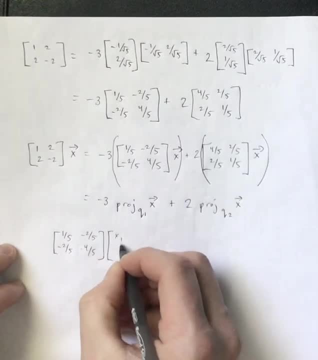 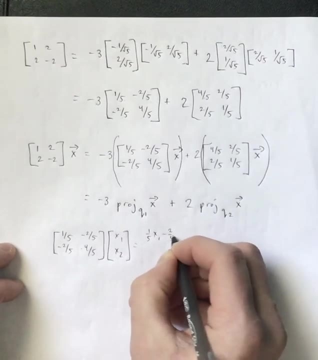 And I'm going to write x As x1, x2.. This is just in general, But you'll end up getting 1 5th x1 minus 2 5th x2.. And then down here, negative 2 5th x1 plus 4 5th x2.. 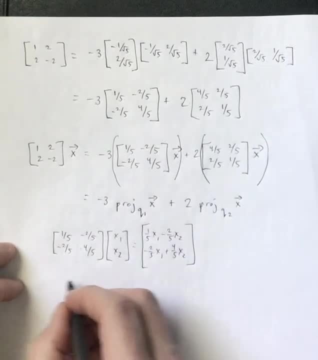 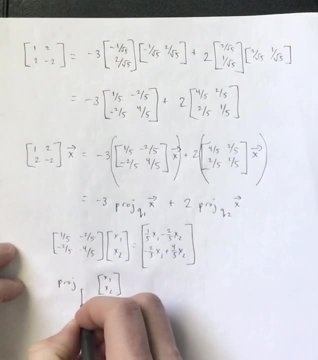 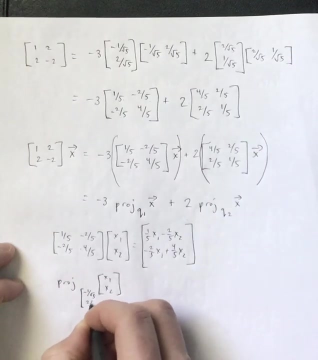 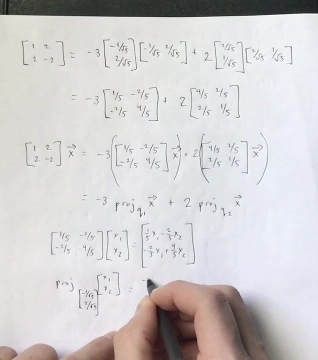 Now to convince you that that's the same thing as projecting, Let's project x1, x2 onto the vector. Let's see q1 was Minus 1 over root 5, 2 over root 5.. So remember that will be the dot product of the two. 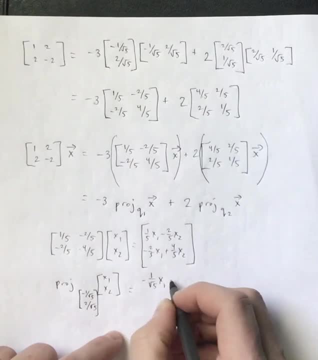 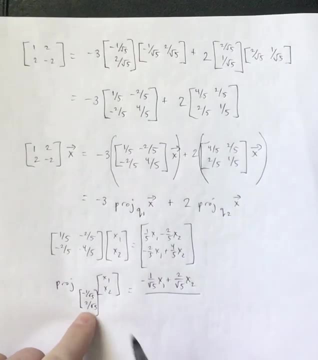 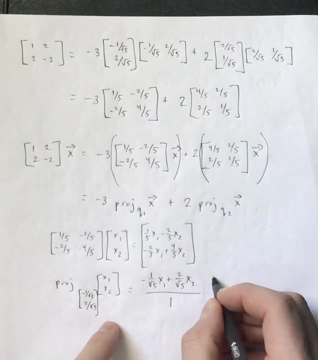 So negative: 1 over root 5 x1 plus 2 over root 5 x2.. Over the dot product of this vector with itself. And remember it was a unit vector, So we're just going to get a 1.. And then we will multiply that. 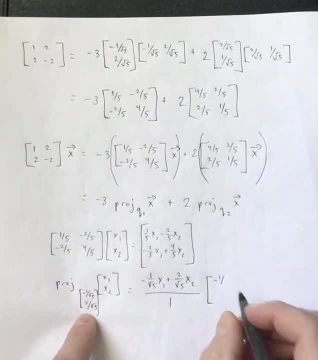 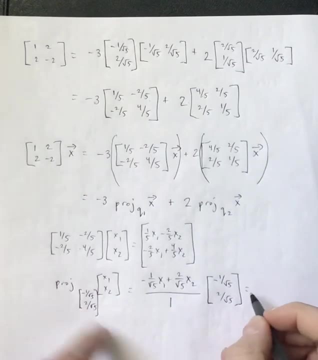 By this vector, That will be the scalar that goes on this vector. And so notice that if I were to distribute this across to both components, I would get 1- 5th x1 minus 2- 5th x2.. And then down here, negative 2, 5th x1 plus 4- 5th x2.. 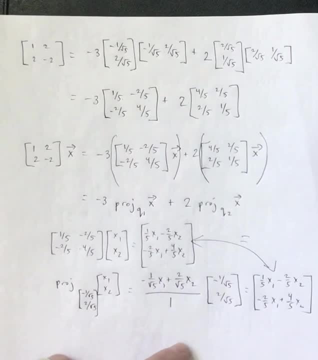 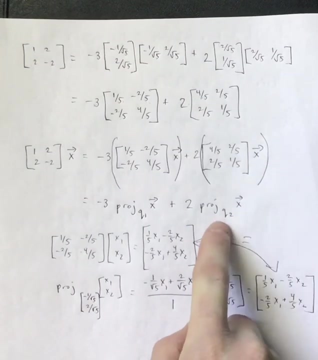 And you can see that that is In fact the same thing that we ended up with when we just multiplied by this matrix. I'm not going to do the second one, but it'll work the exact same way If we were to compute that, except it'll be the projection onto q2.. 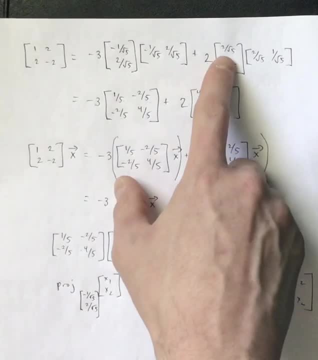 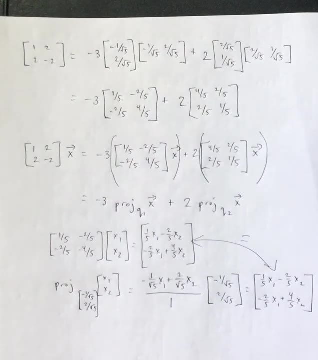 Which, for this problem was here. it is 2 over root 5, 1 over root 5.. So that's what a spectral decomposition would tell you. Not only is it a decomposition, but it's a decomposition Into, essentially, projections. 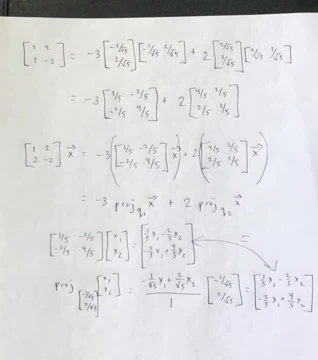 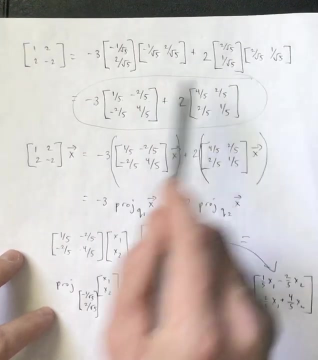 Essentially saying: let's decompose so that it would be essentially applied to a vector, would be in the direction of one of the normalized basis vectors plus the other one. But again, just to recap, this was the answer for this particular problem. 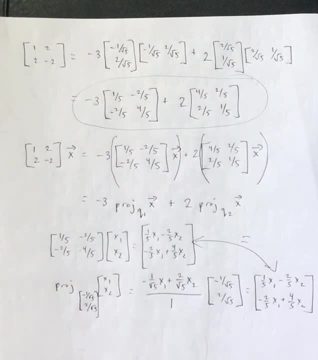 The rest of it was just checking and seeing what that ends up being, So I hope that makes sense And if you have any questions, Please let me know. 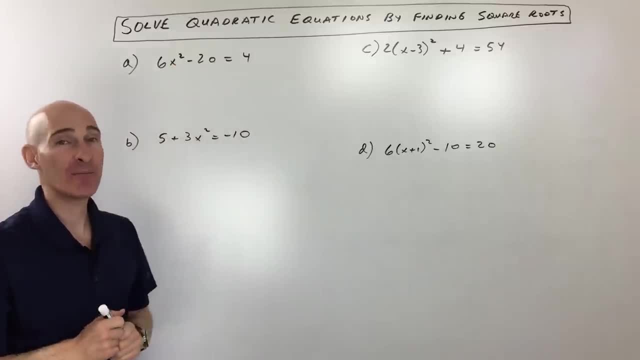 This X by itself. So what we're going to do is we're going to work from the outside in by doing the opposite operation. So what I would do first is I would add 20.. Okay, So, working from the outside in towards X, I'm going to do the opposite: add 20, right? So if I do that, that 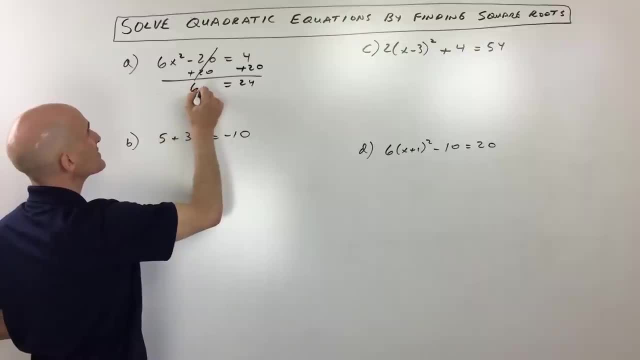 gives us 24.. Okay, These are going to cancel. We've got six X squared left, right. Now, same thing. We're multiplying by six. We want to do the opposite of multiplying by six. We want to divide both sides by six. So we're narrowing down or getting closer to that X, to isolating it by. 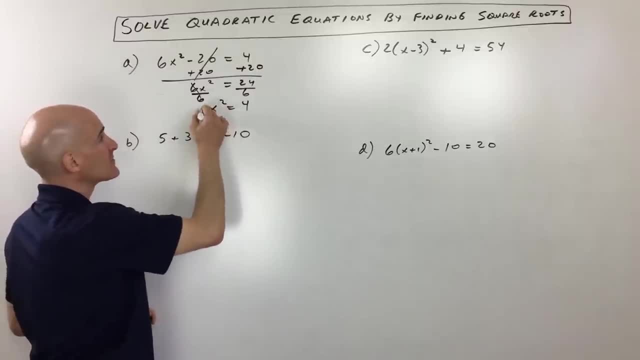 itself. And then now we've got, X squared equals four. We want to do the opposite of squaring, which is to take the square root of both sides. But remember, when you take the square root of both sides of the equation, you actually get two answers plus or minus, and the square root of 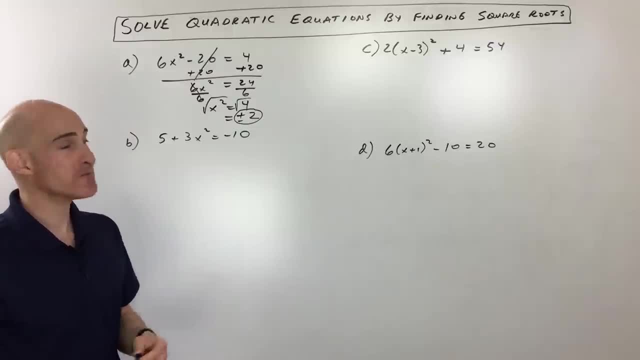 four is two. So those are our solutions: positive or negative, two, Okay. Example B: here it says five plus three, X squared, equals negative 10.. Same idea: We want to work from the outside in towards that X. get that X by itself. So let's do the opposite of adding five, Let's subtract five. 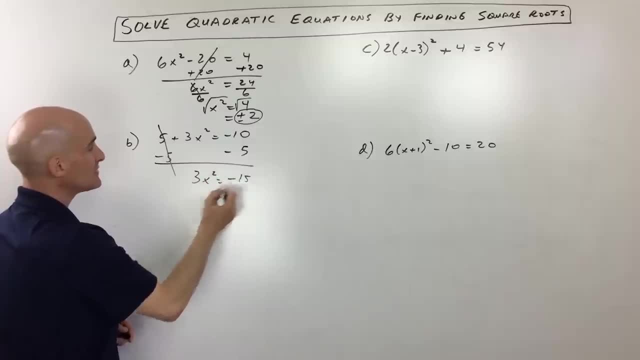 These cancel, We get three. Three X squared is equal to negative 15.. We want to do the opposite of multiplying by three. We want to divide both sides by three, So X squared gives us a negative five, And we want to take the square.